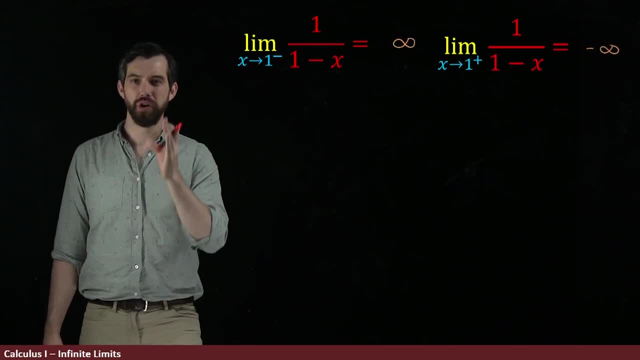 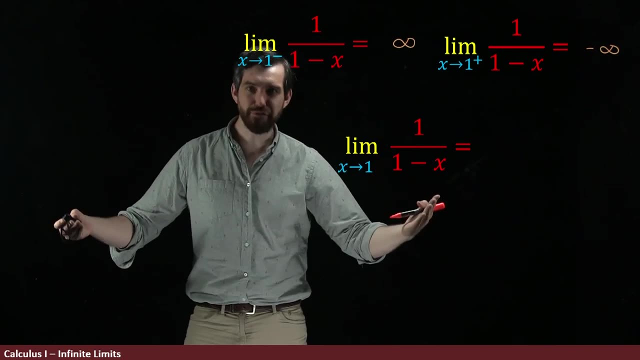 And then, if I want to try to figure out what happens to the limit, the two-sided limit, the one where I don't put any exponent, and what I mean is from the left and from the right, both sides put together well, 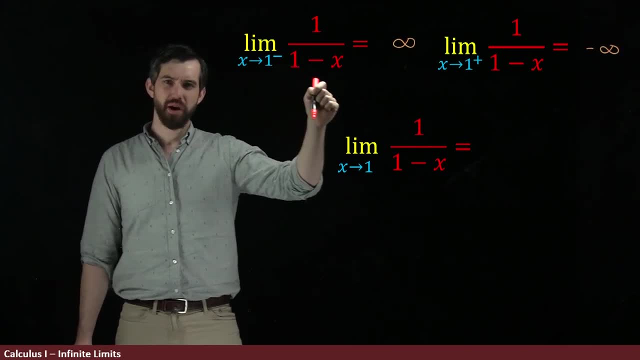 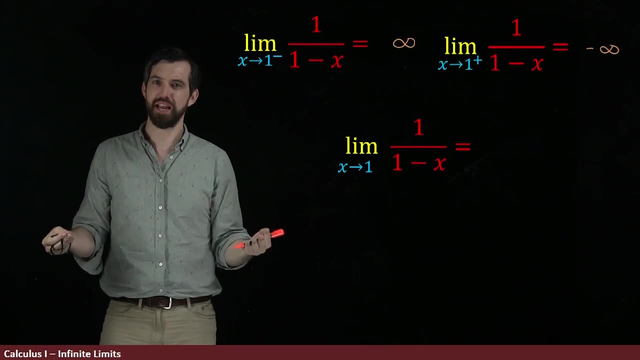 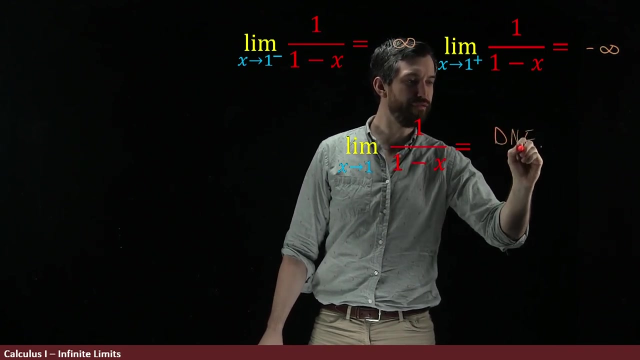 on the one side it's positive infinity, on the other side it's minus infinity. so they're different things. It's not the case that when you come from the left and from the right, that you get to the same result. They're different things, and so what we write here is d n e for does not exist. 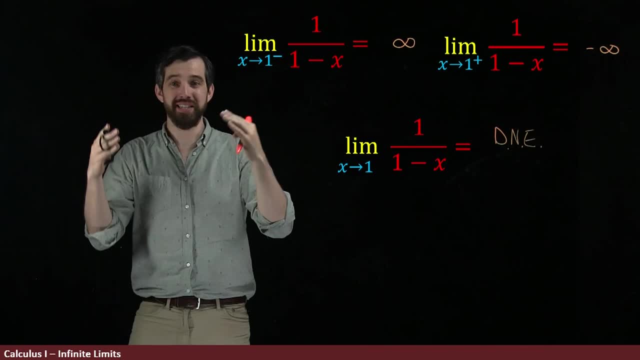 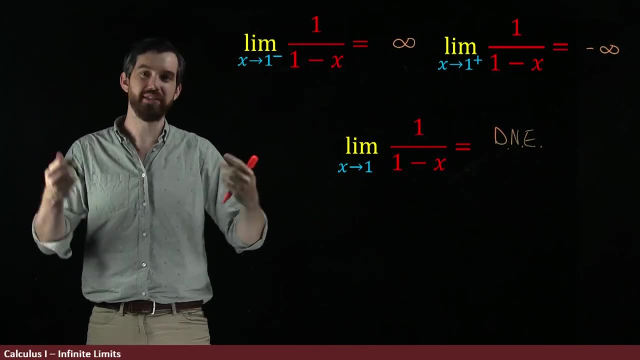 And any time where the limit from the left and the limit from the right go to different values, or, in this case, one goes to infinity and one goes to minus infinity, which I don't think of as a value, it's a concept, but nonetheless it's a different thing. 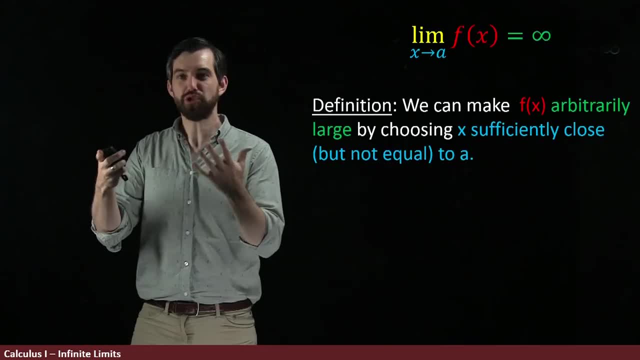 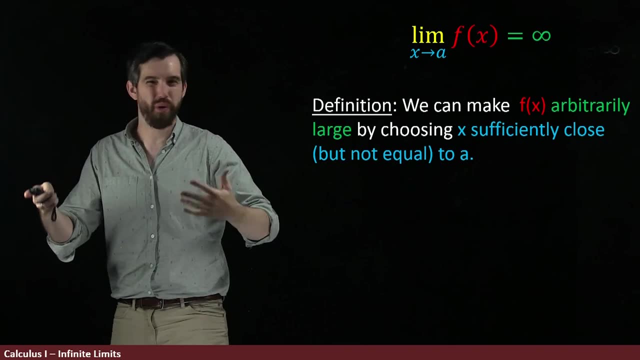 then we're going to say that this limit does not exist. So let's try to define this concept, the concept where the limit as s goes to a, is equal to positive infinity. same, by the way, for minus infinity. you can adjust it. 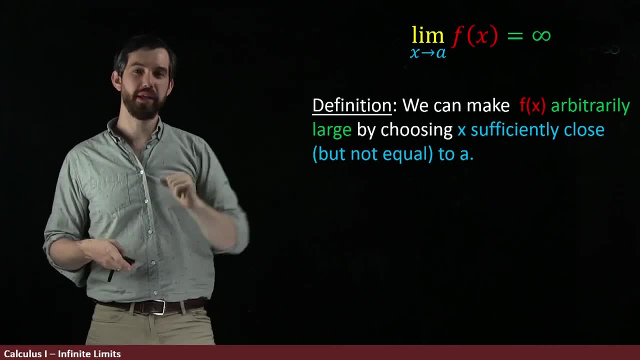 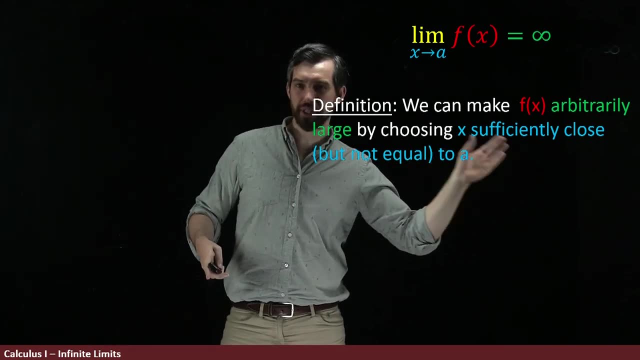 I'm going to say that now my function gets arbitrarily large. a million, a billion, a trillion, however big you might choose. we can accomplish that by getting really, really, really, really close, but never equal- really, really close to this value of a. 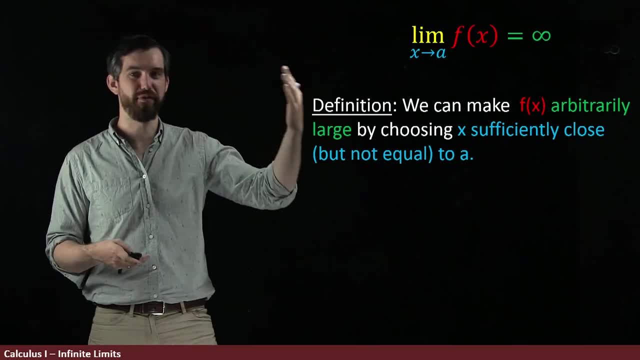 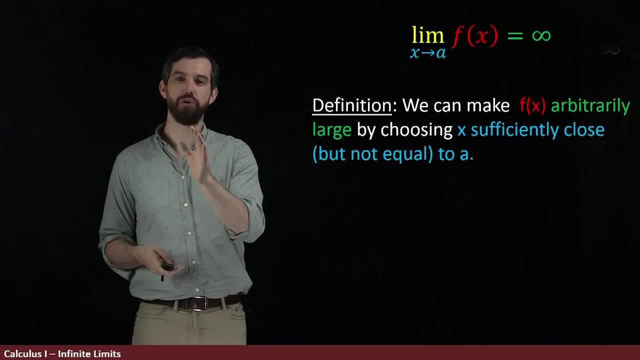 And there's also an analogous concept when you take the limit from the left or the limit from the right- plus or minus infinity. there's a bunch of different versions, but the idea is always the same. I had to make one little quick caveat, which is that when we talk about a limit being equal to infinity- 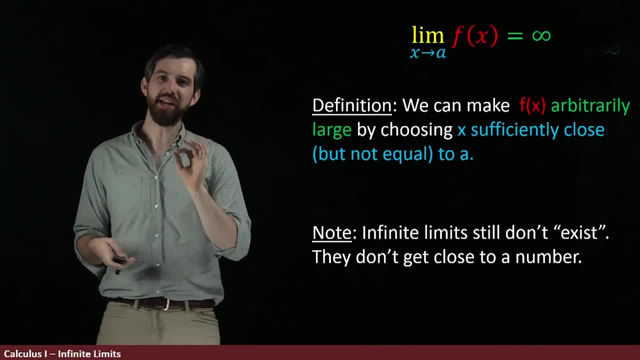 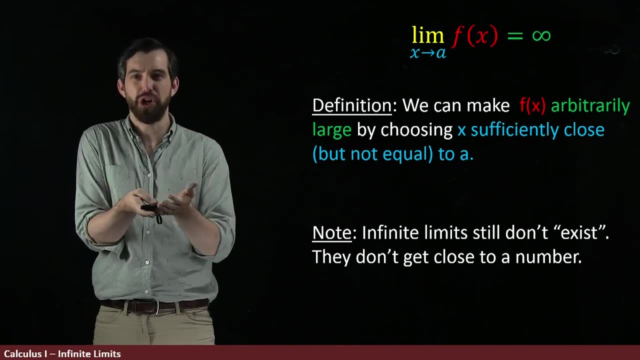 in a sense it's a bit of an abuse of notation. The limit still doesn't exist. It's not like we're getting close to some number. in the way, if I say the limit is equal to 7, we're saying we're getting close to 7.. 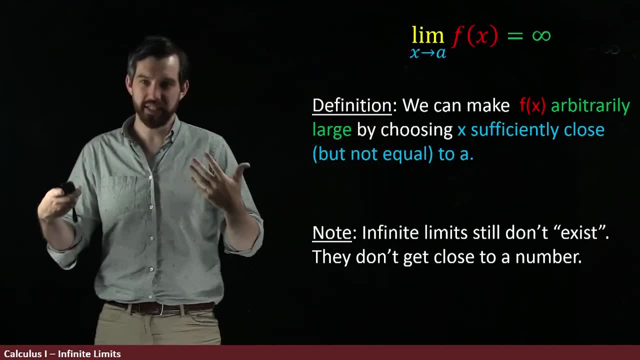 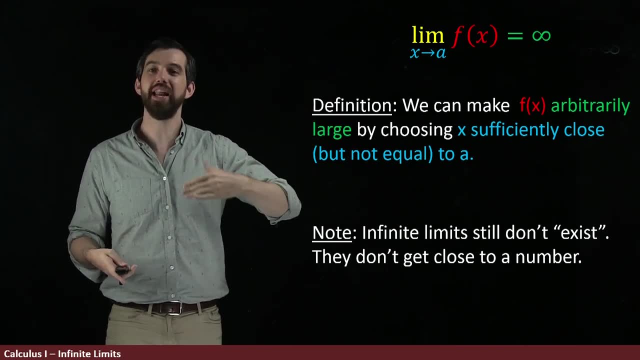 We're saying we're getting close to some number. So this limit doesn't technically exist, but among all the limits that don't exist, that the infinite limits obey this particular property of getting arbitrarily large. So the convention is going to be that, if I ask you for what this limit is, 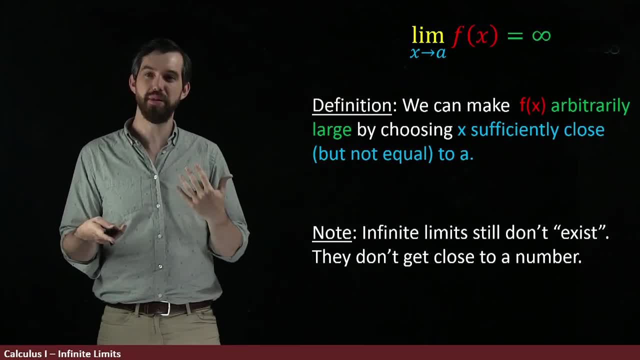 you could say that it's equal to infinity, but you maybe note in the back of your mind that that doesn't mean the limit exists. it doesn't get close to any particular number.